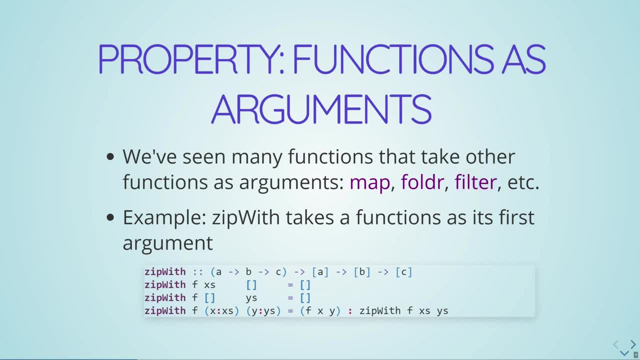 because they took another function as an argument. So another example is the zip whip function. Let's take a look at this function. So zip whip, it takes a function f as an argument. So you can see in its type signature how we bracket around the first three arguments. So we're saying the. 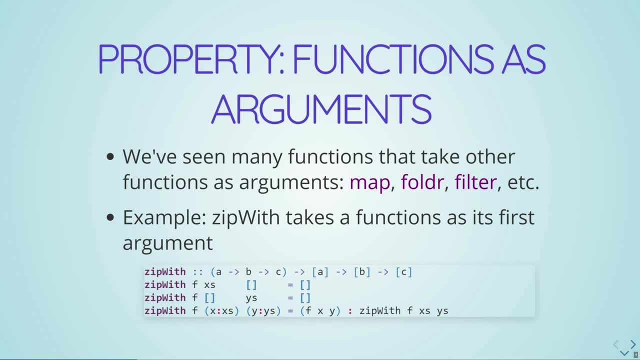 first argument: f is actually a function in of itself that takes an a and a b and then returns a- c, okay. And then it takes two lists, a list of a and a list of b. What it does is it takes this f and the first elements of each of these two lists and it applied. 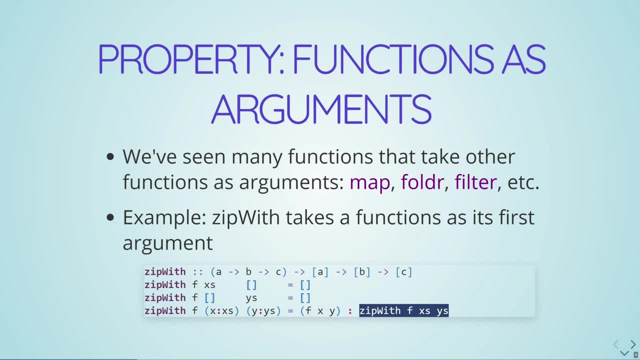 f to those first two elements and then continues building the list, So it kind of it goes through the list. It's like zip instead of. but instead of zipping each element of the argument together into a tuple, it zips it together with whatever function you give it. 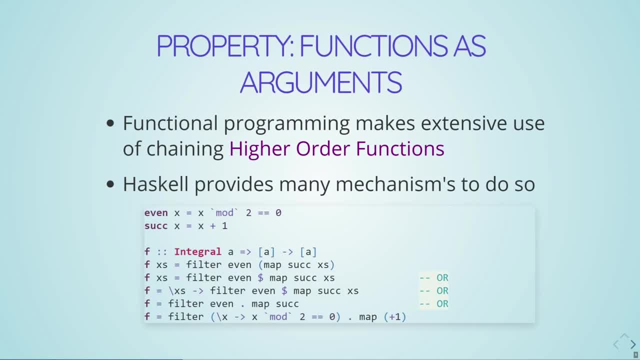 f here. okay, So functional programming- it's in the name: functional. In general, we make extensive use of functions and in particular higher order functions, because higher order functions are functions making use of other functions in a very special way, And Haskell. 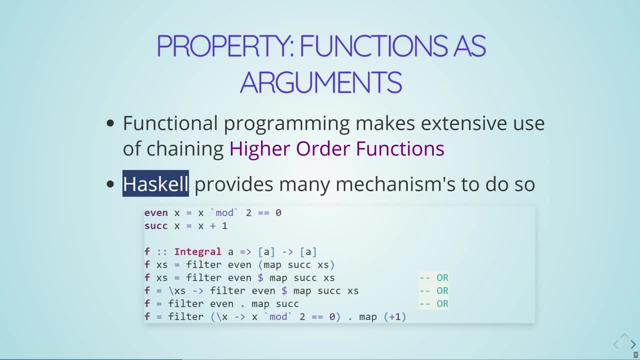 as language provides many mechanisms to work with these higher order functions. So consider some functions here, like f here. okay, f is going to filter out all of the even elements from mapping the successor. so plus one to a list of x's okay. So there's a number of. 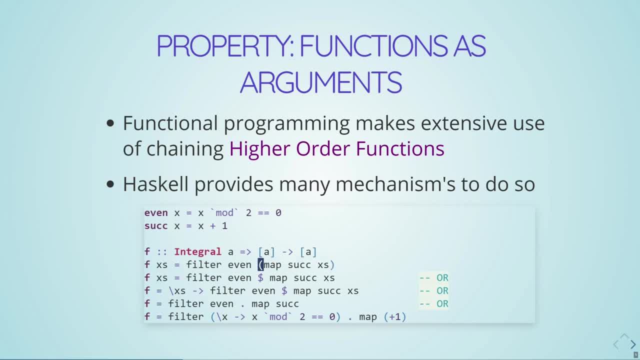 ways that we could write this. We could write this like this: or we can get rid of these brackets with the dollar sign, which is a combinator that we'll go over in a bit, Or, instead of explicitly okay, specifying the argument in the function definition, here we can write: 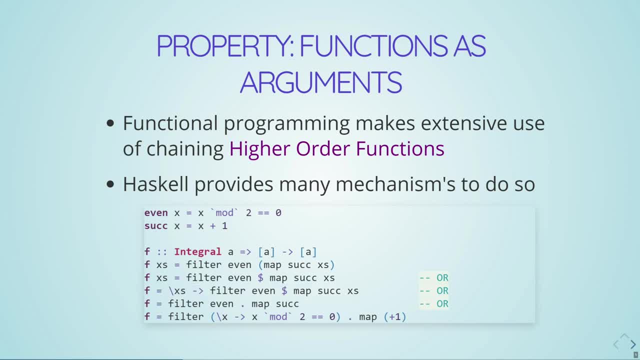 it inside of a lambda expression here. Or we could compose these two functions together using the dot- here This is another function combinator that we'll go over a bit- Or we can use a lambda expression instead of using these predefined functions. okay, So instead. 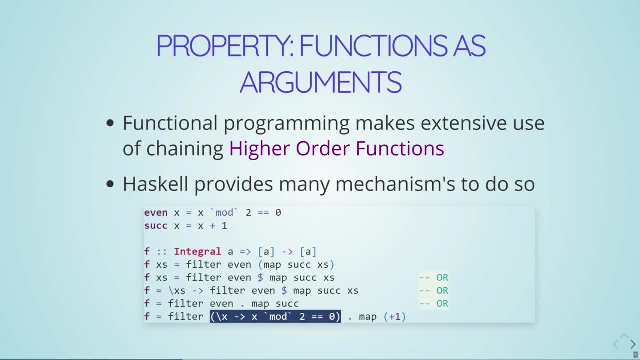 of writing even here we could just put the even Evidence that we are going to GetLambda And this is the end result. So we could do some real-time code into a lambda expression And instead of writing successor here we could do this just with plus one. okay, So there's a lot of different ways we could write. 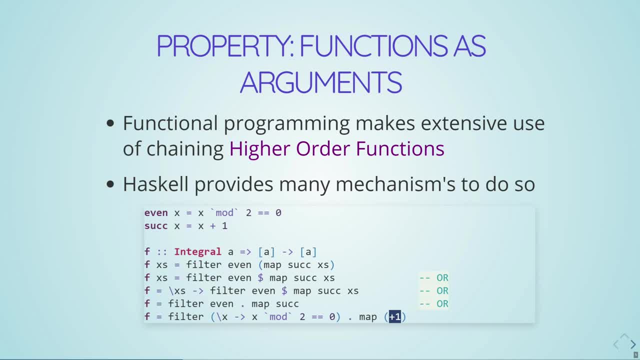 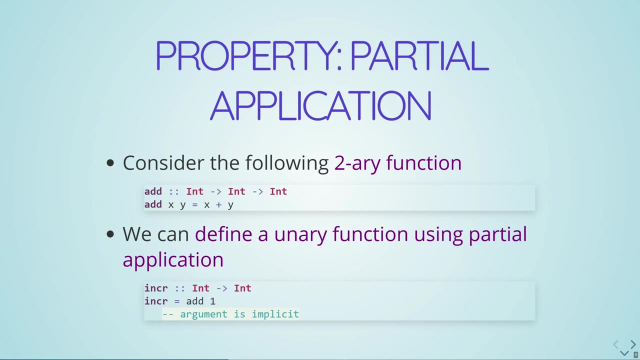 the same sort of functions in Haskell, because Haskell gives us so many different mechanisms for manipulating how we write functions, And today we'll discuss a variety of these mechanisms and when you might want to use them. So let's discuss another property of functions in Haskell. 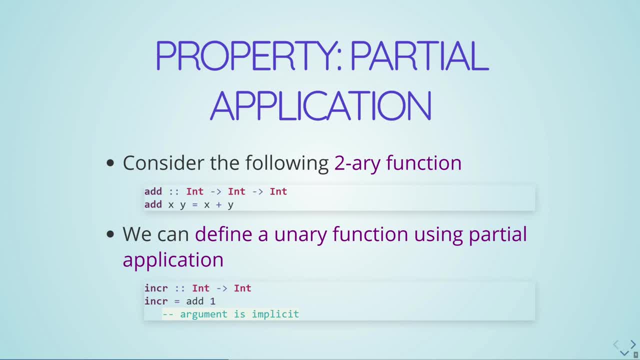 application. So this actually has to do with currying how we define functions, which we talked about before. So consider the following two-ary function. So recall, the arity of a function is just the number of arguments that it takes. So a two-ary function just means that. well, 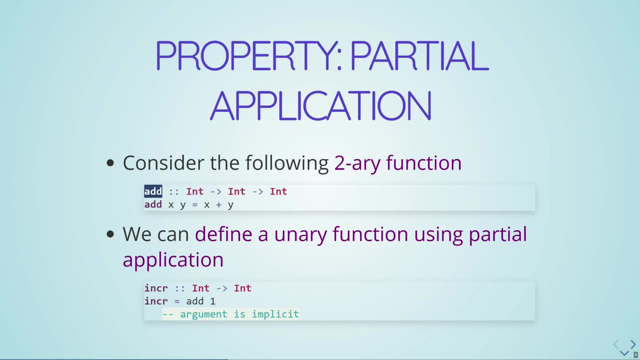 it just takes two arguments to it. So add here takes an x and y and it just adds them together. So if we wanted to, we could define a unary function. okay, unary meaning one-ary is the same thing. So unary just means it takes one argument using partial application. So this is: 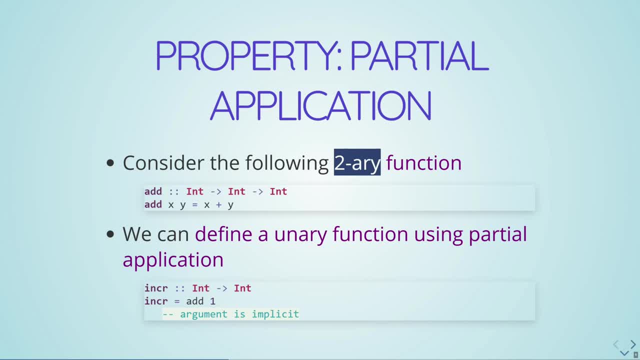 another consequence of having first-class functions and having currying that we can just say: add one. okay, we could partially apply it. we could give it one of its arguments and add one return- It returns a function, Okay. so if you give it just the one argument, it returns this function. 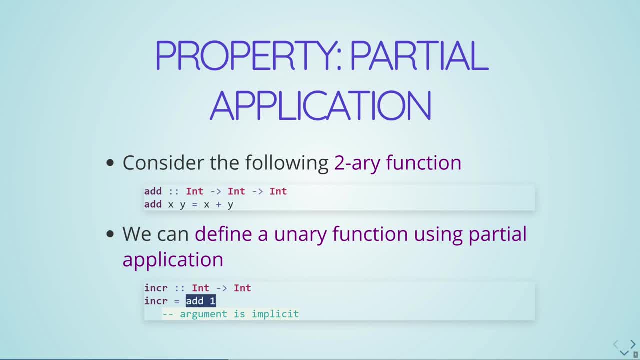 here int, int, okay, And then we could write: increment here is equal to this And you'll notice increment here it doesn't. it doesn't show an argument. There's no argument at here, but it does take an argument. it takes an int and then returns an int. So the argument: 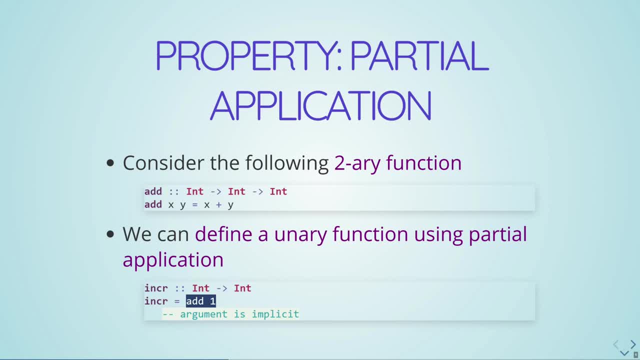 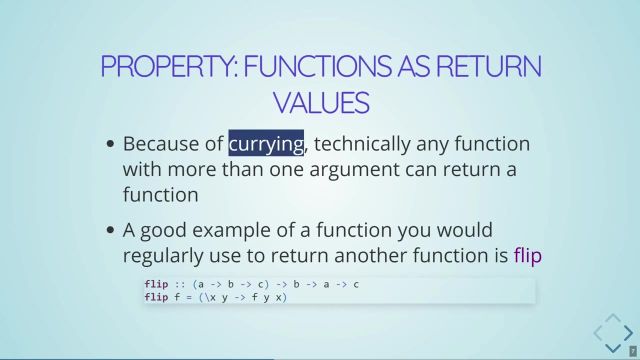 is implicit because it's add one. it returns a function and then we're assigning increment to it like we would assign to a variable. So there's an implicit argument here. So if we look at the consequences of this, basically because of currying and partial 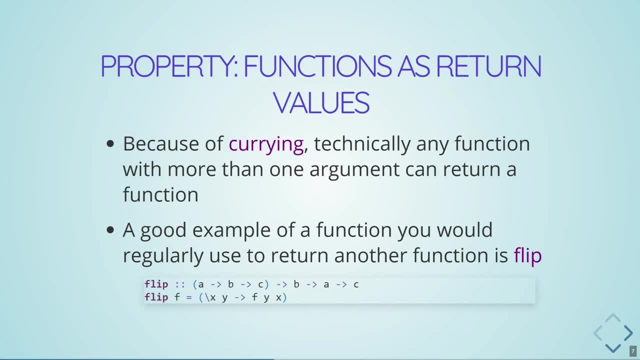 application. technically, any function with more than one argument you can look at as returning another function. you can view it that way. as it returns another function, you at least have the option of it having returning another function- A good example of a function you would regularly do. 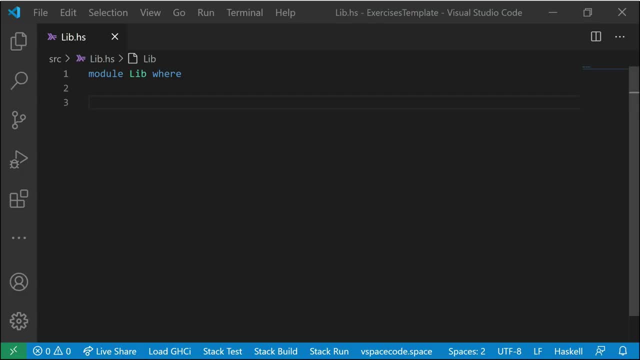 this with is a function that returns another function. So if you have a function that returns another, flip would be the flip function. So flip the way you define it. so clip it would take a function as an argument. so an a and b goes to C. so this needs to be a binary function And 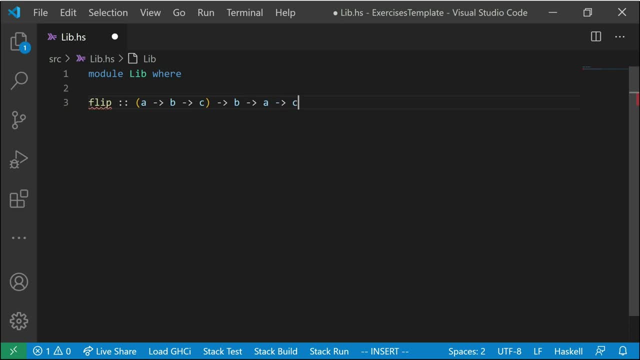 then it basically takes a B and an A and then goes back to C. So it's gonna. it's gonna flip these arguments around. Okay, so you could define it using a lambda expression. say: take an x, y, And sorry, it's gonna take. 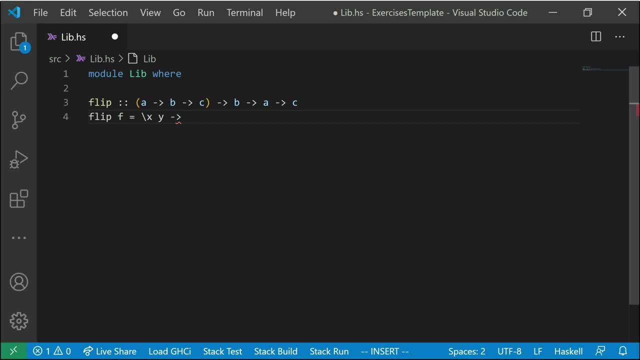 and f as an argument, and then it's going to return a function, this lambda expression that takes- we'll do it this way- a y and an x and applies f, x, y. okay, so it's going to take the arguments to this function in a different order here. okay, if we look at how this might be used, you could take, let's say, 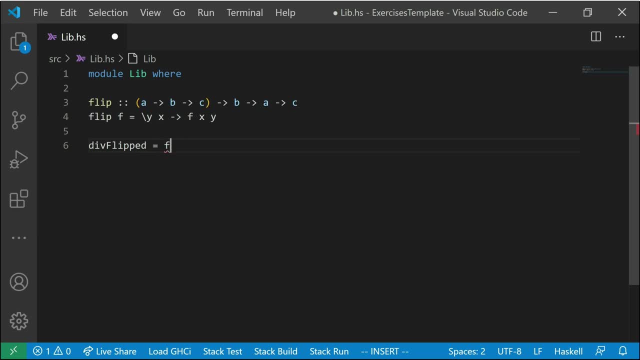 div flipped and we could flip around division. we can say flip and give it the division operator and we actually need to call this. there already is a clip. this is a prelude function, so we'll call it flip prime. okay. and if we look at how div flipped works, if we now open up a terminal, 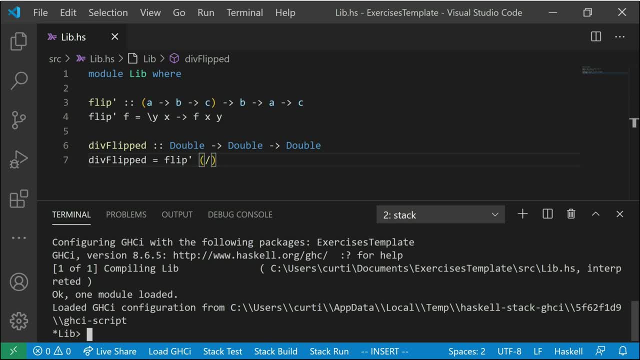 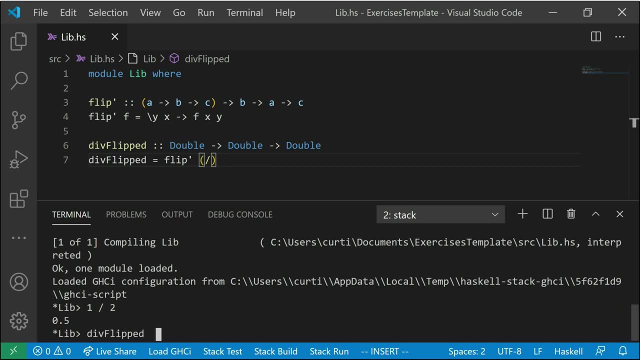 okay. so of course, something like um one div two is 0.5, but on the other hand, div flipped one two, okay, it's 2.0. so it's doing the opposite there, right, so we, we can now um give uh div, let's say, let's say we had a. 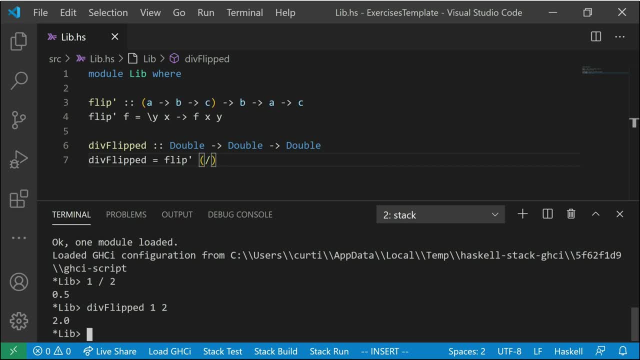 list of things and we wanted to divide everything in that list by two. we could say something like map, give flipped two to um list of four, six, eight, okay, and it's going to divide everything like two like this, and we we could have even kind of skipped the two part. we could have said flip div and not even defined our 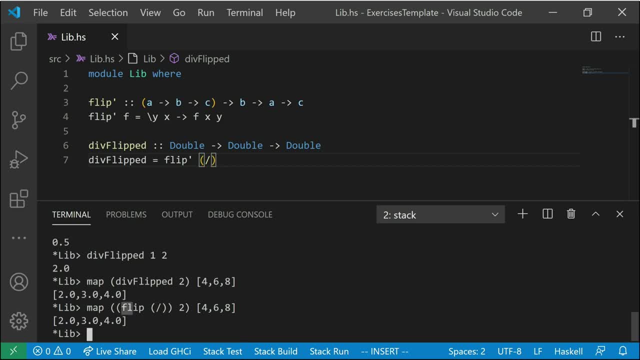 own function fully here. and this would work the same way if we do flip div and we kind of have a bracket to solve to be like, okay, this is whatever this is returning, okay, this returns a function, and then just use it like a function. so this is another example of how functions are first class. 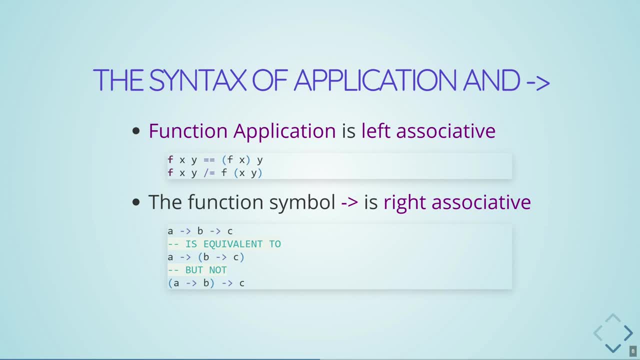 in haskell. now, in talking about how functions can take functions as arguments and return functions and how that's conveyed in the type signature, it's important to notice the syntax of that operator. we use inside the type signature that kind of arrow operator, so function application is left associative. that means when i call a function f of x, y- okay, these brackets here. 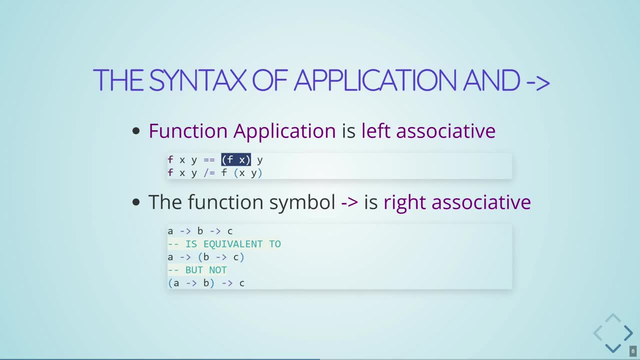 are implicitly there. this is, this is implicitly always happening. okay, um, so this is not what's happening. this is what's happening. there's always this bracket here, and if there was more arguments, would be another bracket here that you would see. on the other hand, this arrow here is right associated. 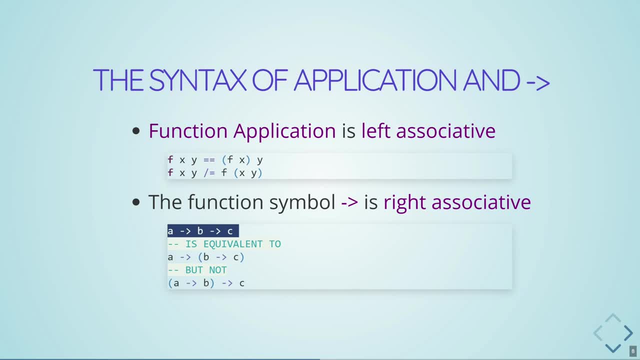 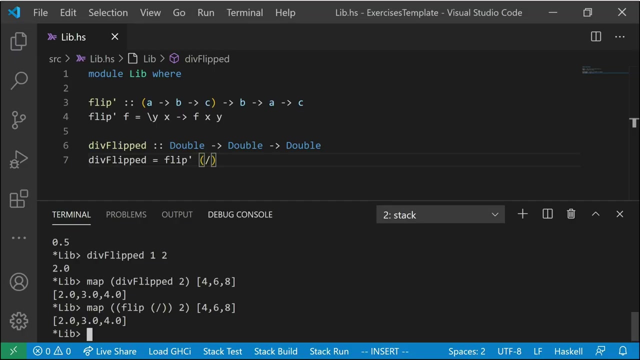 so this a goes to b, goes to c is implicitly the same thing as a goes to bracket, b goes to c, but not this. when you do this, okay, when you put the brackets um, on the left associativity side, that means that you're taking a function- a goes to b- as an argument here, okay. so to relate this to: 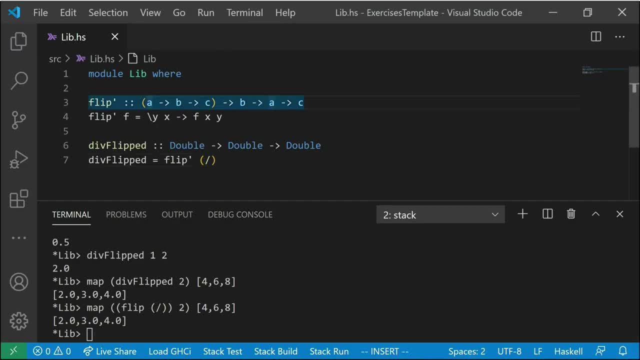 our flip example. so flip here. if we look at its title, signature there's implicitly, so this type signature is the same thing as this, which is also the same thing as this. so this that's what it means for this operator to be right. associative is that these: 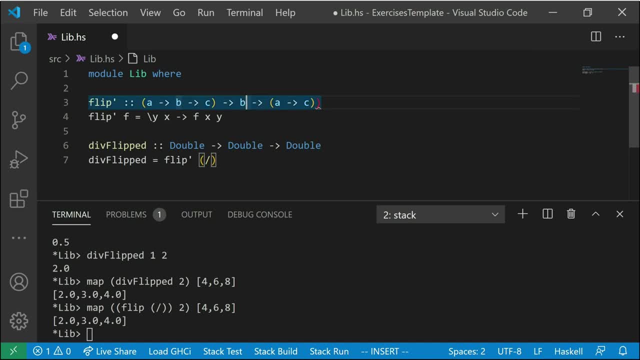 brackets are just kind of implicitly there, even even if i don't put them there. that's how the precedence of of this expression is being evaluated, right? and when i call um f of x, so even if i have some function, f, x, y, the m equals. so, baby, all add up together right? 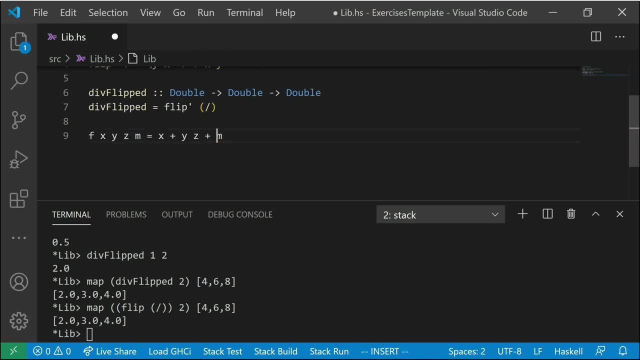 okay, this function if i were to call it later, so if i were to create some variable, add some stuff, i would call f one, two, three, four when i'm calling um f one, two, three, four. here this is actually the same as me writing f of one and then that returns a function. 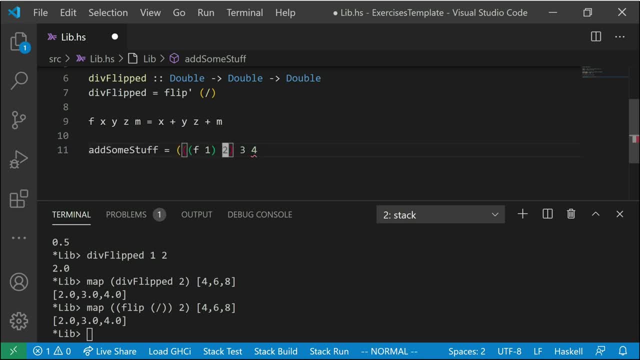 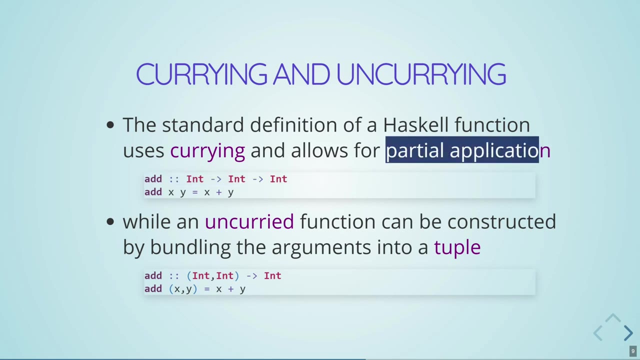 which then you call two on, which in turn returns another function, then you call three on, which in turn calls another function that you then call four on. and just a reminder once again, i keep bringing this up, but this partial application really comes down to the feature of currying, okay, this idea that a function returns another function. and if we wanted to, 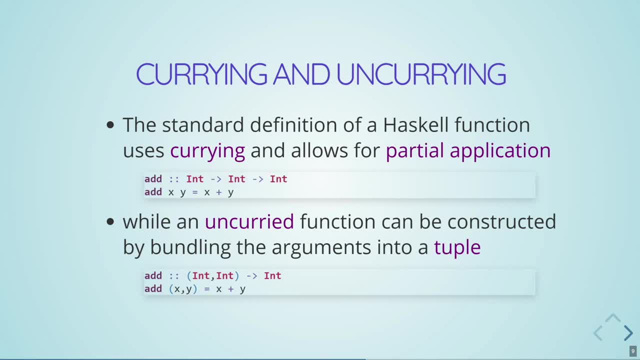 uncurry something. essentially, what we do is we wrap it into a data type, the standard one being a tuple. so if we wanted to make sure that both of these arguments, like, let's say, x and y here, they're always given together before the function can be, 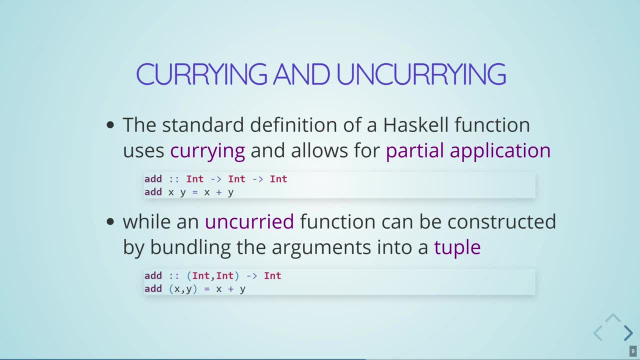 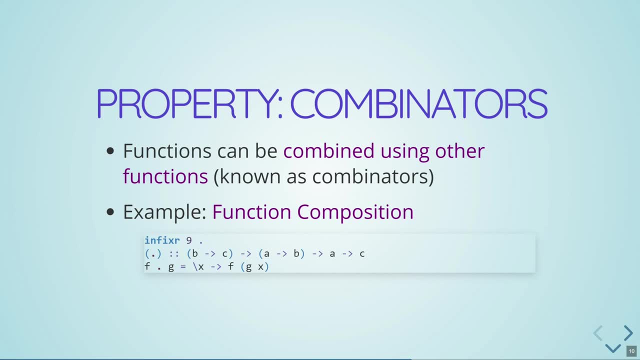 applied, you wrap it inside of a tuple. now let's talk about a important feature that having these higher order functions gives us, which is function combinators. so we could take these functions that use other functions as arguments and use it as a way to combine functions in. 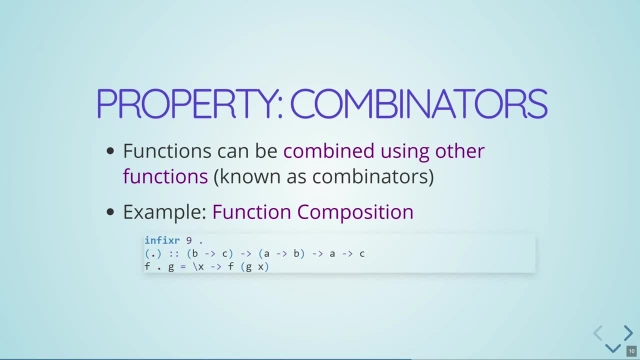 particularly interesting ways. so a very standard function combinator would be something called function composition, which might be something you recognize from mathematics. so we use the dot operator to express function composition and basically what we do is we take a function that takes a- b and returns a c and another function that takes an a and returns a b. okay, and then 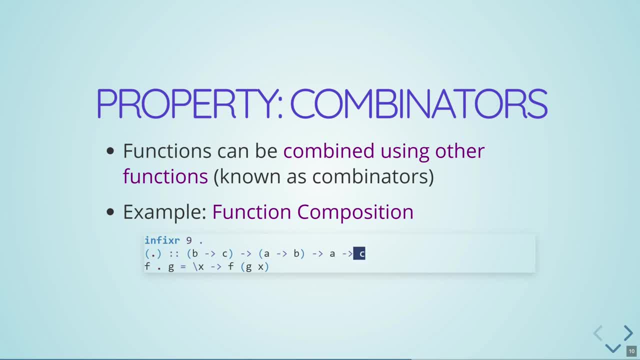 we take an a and then return a c. so basically what it's doing is it's kind of chaining those functions together. so the simple way to define it is we take that a value, okay, and we apply it to our second function, g here. so g takes an a and returns a b. 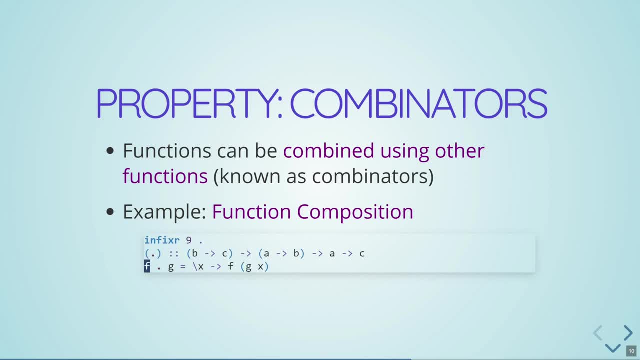 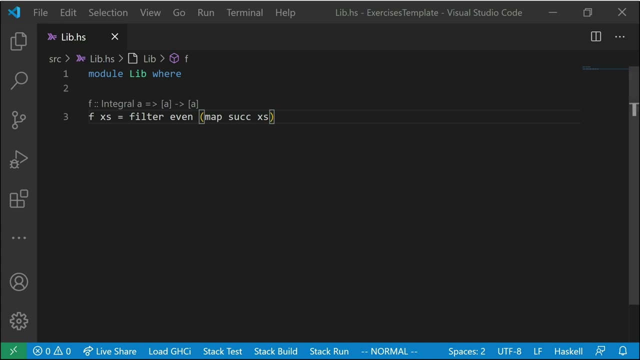 okay, so this returns a b value. and then our first function, f, here that takes a b. so it's going to take the output of this function and then return a seed, which is what we turn in the end here. so this way we could compose two functions together. so as an example of 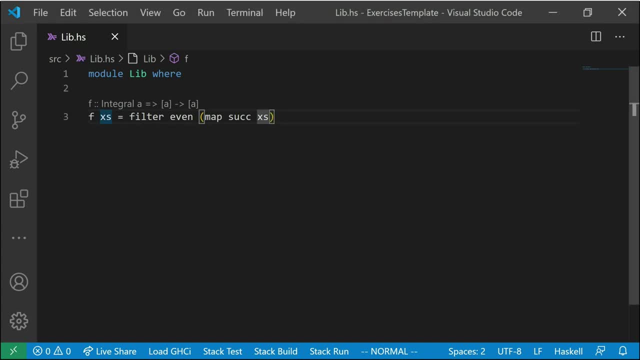 function composition. let's go back a second to that example we had before, where we had this um even function and successor function, which should really be defined like this, is plus one. okay, and what we're doing is we wrote this function, it goes over a list, it adds one to. 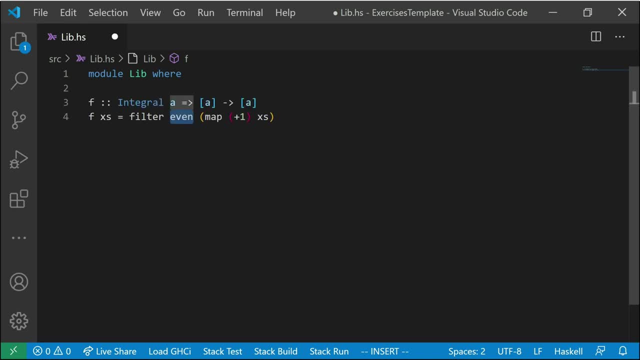 everything, and then it takes only the even values of that list using filter here, right? so another way we could define this okay is we could have said: well, this function, this filter, even function composed of map plus one, okay, and then we don't even have to actually. 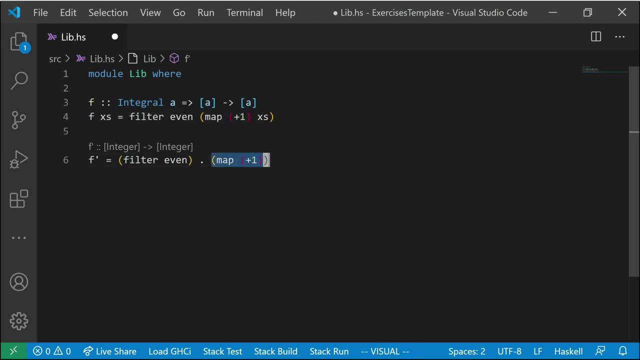 put our argument here. so this is: this is one function composed of another function, so this returns another function, f here. okay, so it's the same. it's actually the same function it gave. it gave me a different type signature here, but it is the same function. let's go a. 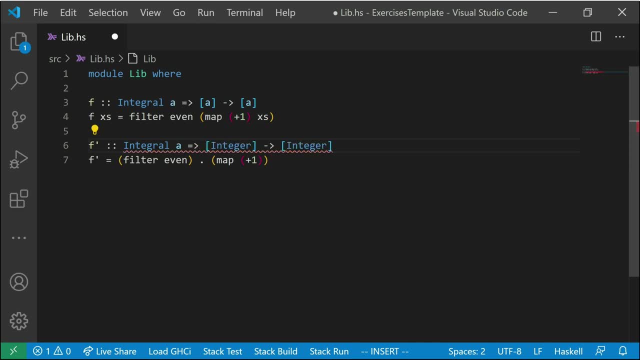 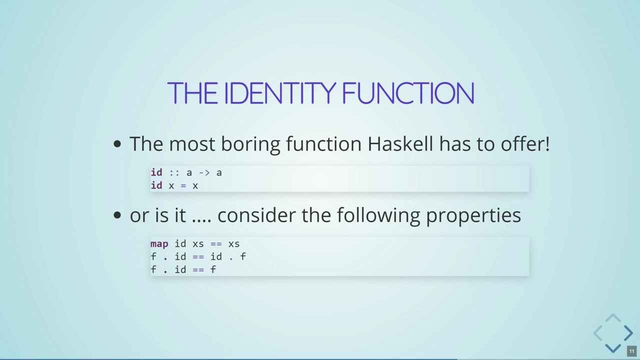 okay and then use that instead of okay. so this is actually a particular style of writing functions that's actually known as point free or before I go on to show you more common areas, let's point out another interesting, or perhaps the most boring function that Haskell has to offer: the identity function. so the identity. 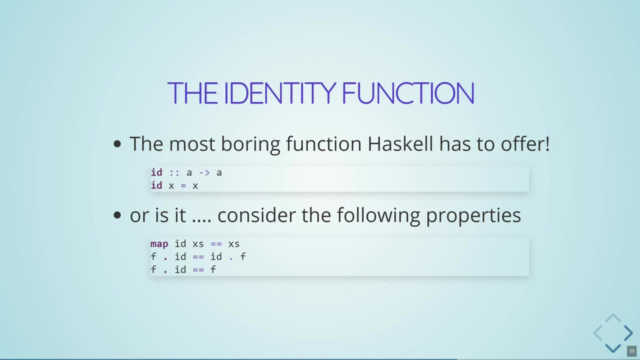 which we usually just write, as it is a function that takes an x and returns an x. it just returns the exact same thing, so this seems like the most useless function ever in terms of actual practical computing kind of is. however, it's kind of neat to consider the properties that you could define using the 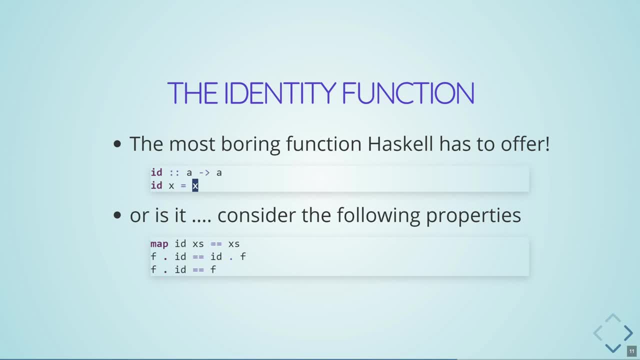 identity function. so we wanted to define some properties that say map should hold. so you could. you could define map, like I showed you, over other data types and if you wanted to find a common property that map should hold, one of them should be that mapping the identity over the list x is will return that same list x's. so what does this mean? this? 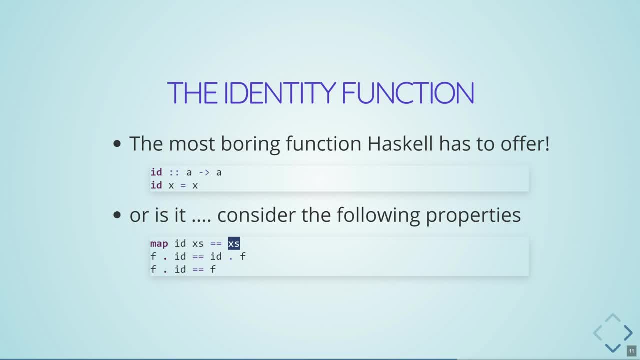 means that whenever you define a map function, it shouldn't be like changing around the structure of the list or whatever data structure you're working off of arbitrarily. it shouldn't just be like changing things around. what it should be doing is it should be going and applying the function to each element of the list right. so for each element of the list right, the same factor that there is in order to find a common link value is defined for any type. so, for instance, if I had a function with sort i as log x, here we can just change the identification. so what would population Card? 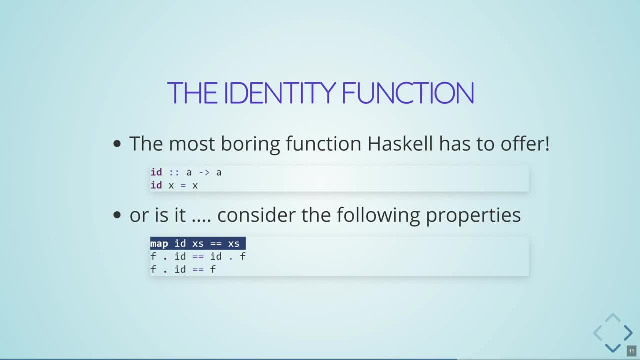 right. so this gives you an idea of like. okay, this is some of the expected behavior out of map. this also gives an idea about how the dot works. okay, so if we have a function f and we compose it with id, that should be the same thing as composing id with f and, in fact, having a function f composed. 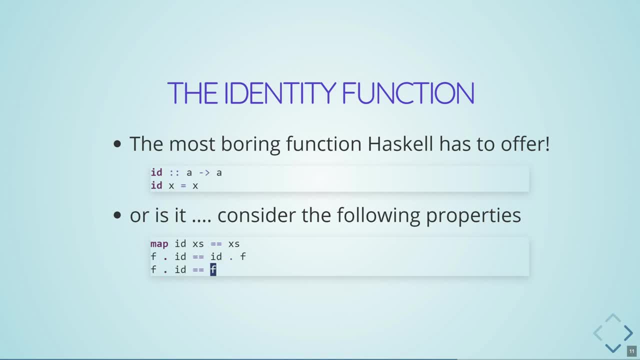 of it should just be the same thing as if in general. so if you're interested in defining properties for how certain functions, particularly function combinators, should work, this identity function is actually pretty useful for that, and this is part of the reason why, if you study functions from a more theoretical mathematics background, you'll talk about the identity. 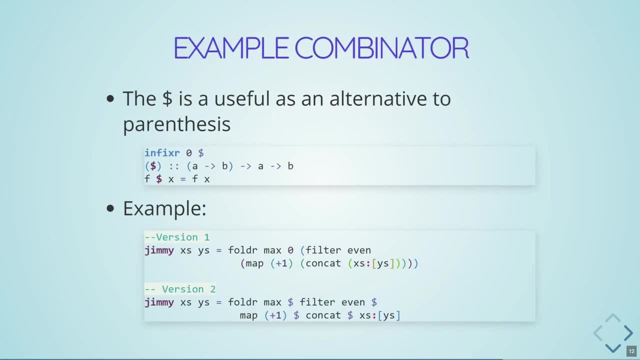 function actually all the time. so let's talk about another example: combinator, here. so the dollar sign combinator is a very useful alternative to properties for how certain functions particularly function, combinators should work. parentheses. so it's a bit of a weird definition. at first you're like: why would i ever define? 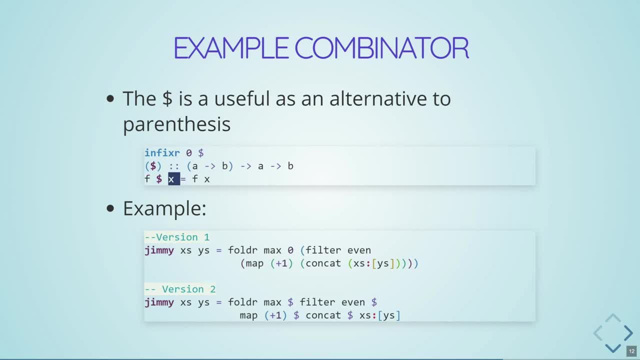 something like this. so it takes a function f and an argument x and then just applies that function f to x. now the trick is it's taking advantage of the associativity of function application that we just talked about before. so remember, i just mentioned that function application is going. 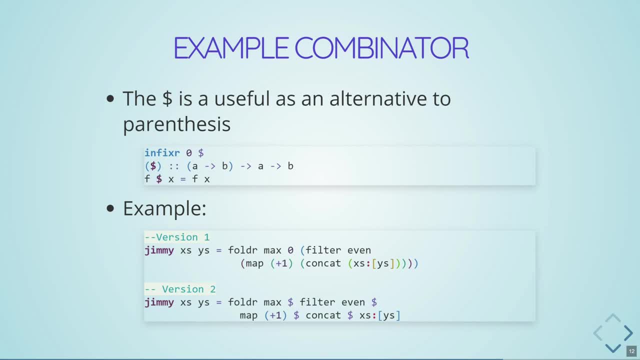 to implicitly put brackets. okay, that associate, um, do the left hand side there. so when you do this, okay, essentially you're getting brackets, you're bracketing stuff. so this allows us to take a function like: consider this first function, jimmy. here the first definition of it. 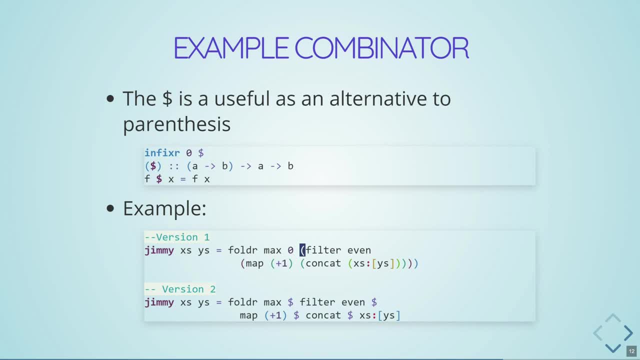 where we're constantly we're applying fold art to another thing and we need to put brackets around this whole thing, and then we're applying again to another function and we need to apply brackets to this whole thing, and then we need to apply brackets to this whole thing and at the end we have this: 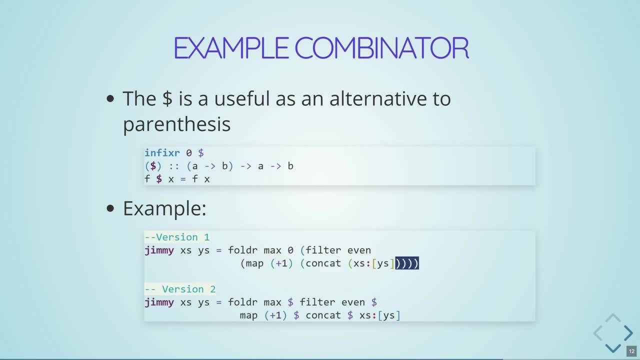 build up of brackets which you get kind of annoying. a lot of you probably um are used to at the point now that whenever you do this you wind up, you know missing a bracket at the end here a lot of you have had this experience, most likely so far, where you miss a bracket and you're going around and 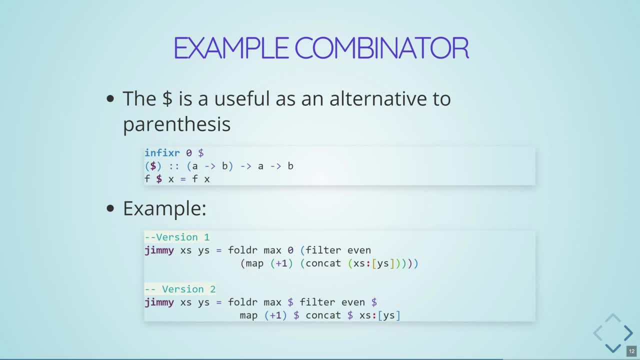 you're counting brackets to make sure you have the right number, so we can use the dollar sign to overcome this. so instead of putting this first bracket here, we just put dollar sign here, and essentially what this is going to mean is that everything that comes after the dollar sign is going to become this x here. okay, so we could. 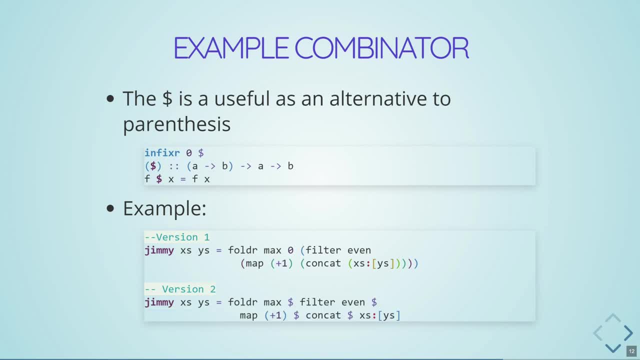 bracket instead of this bracket. we can put a dollar sign here. instead of this bracket, we could put a dollar sign here. now we can't see these brackets here. we can't put a dollar sign here for this bracket. why? because if we did, it would mean that the bracket would continue until the 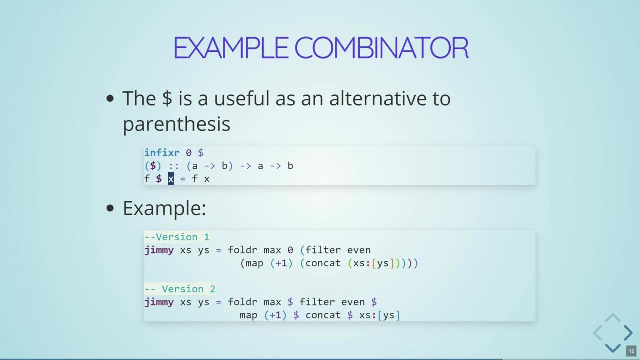 end right like it's, the dollar sign is literally just saying: whatever comes after this, the whole thing becomes bracketed right. so we can't do that, because we don't want everything after this opening bracket to be bracketed. we don't want this whole thing to be bracketed. we. 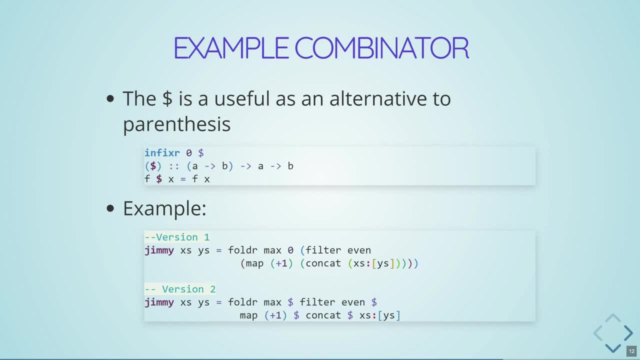 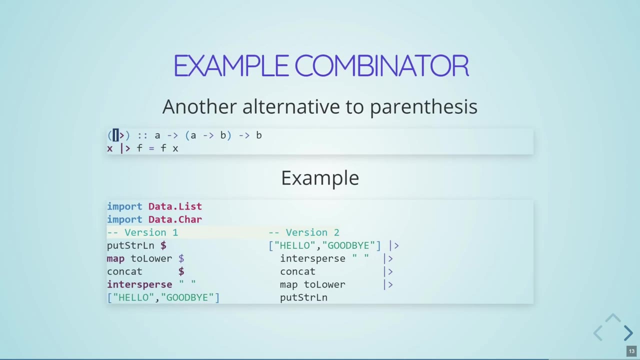 just want this part, so we couldn't put a dollar sign here. but the rest of these brackets we can. okay, and that that'll stop this build big build up of brackets at the end there. another alternative to the parentheses that we can make is: um, this isn't predefined, so we're. 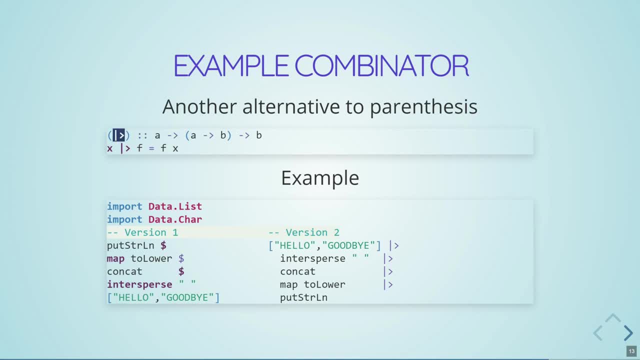 going to have to define this ourselves in haskell, although i kind of think that it should be predefined. we could rate it as this vertical bar arrow thing. i would call this a pipe because it's it's doing the essentially the same thing as the pipe operator in shell scripting does, if any of 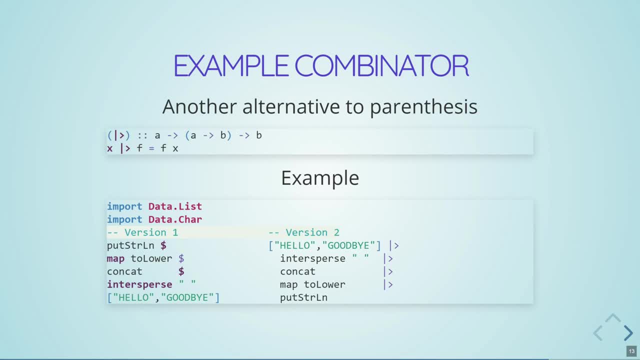 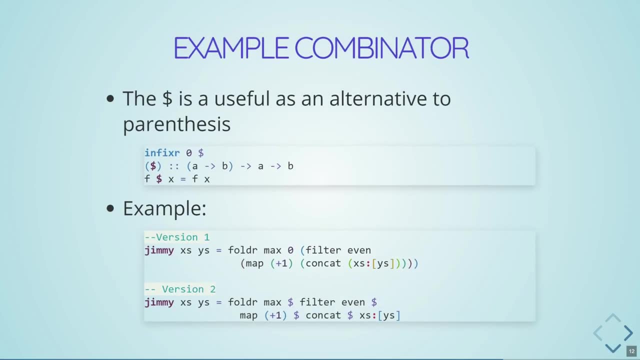 you have ever done some shell scripting before, you'll be very familiar with it. but for those that haven't, don't worry, i'll explain right now. so this pipe thing is kind of like the dollar sign, but in reverse. so the dollar sign takes a function and then an x okay, and it's kind of wrapping brackets around everything on the right. 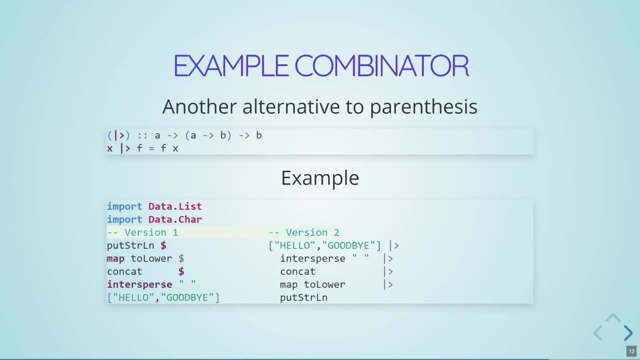 of it right. the pipe, on the other hand, is going to take the x and then the f, so it's kind of saying like bracket everything on the left hand side and then feed it into the function on the right. so to look at example of this, let's say we had a function that's going to print the map of two lower 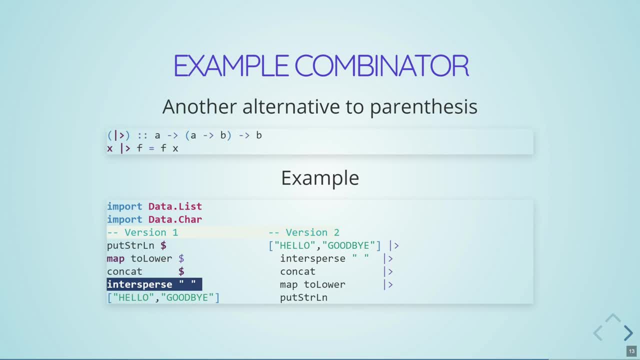 spaces. right, we're going to do this math, the math that we just only have five for both, right. and then the function of this kind of quarter space is going to be masked between one and the other kinds of where, each, and so when we validate this information- so takeіти에게- is when we 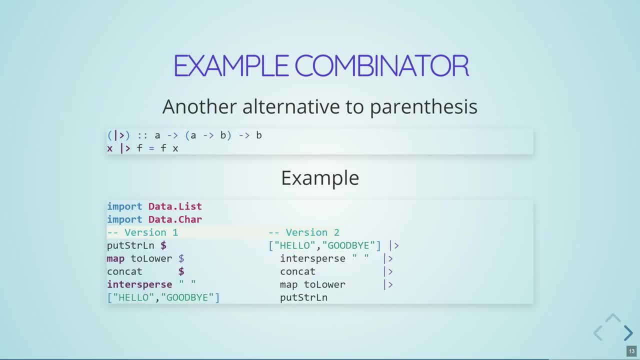 look at this matrix as well, transformed it over into a new hurting level. so now that's extremely important because collaborations are happening right and exactly what i've been doing in this scenario. so it's a one to one500 and one real problem that we have haskell's method. that's really busy. um, let me go over here just for the 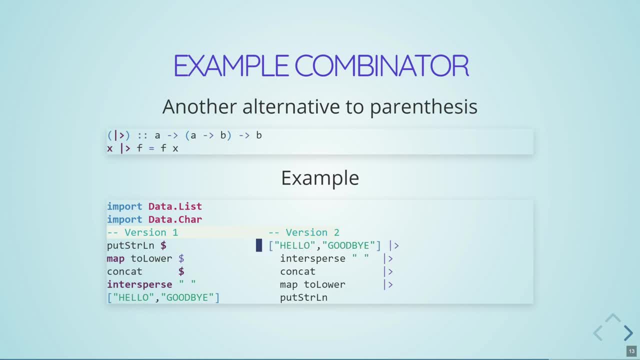 concept essentially encompasses something and you can set particulars and you can set myself a number of yourself here, in my opinion, is kind of better. so you have, you start off with the list and then you're saying intersperse it, and then you're saying inter cap, it can cap. 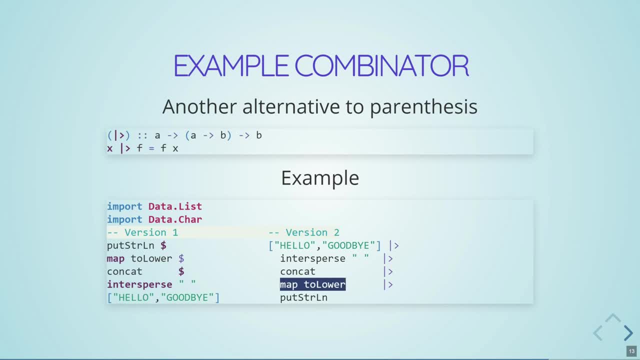 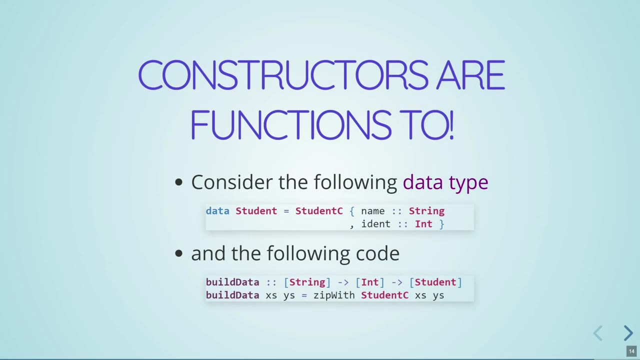 that, okay, put it all together and then turn everything into lowercase and then print it. so it's kind of just two ways of looking at things. you kind of move in like a top-down or bottom-up sort of way of evaluating this. finally, before we finish off, it's worth mentioning that constructors for data types okay. so when?